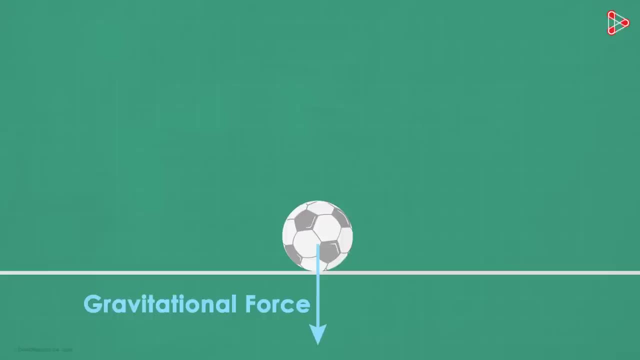 towards the centre of the earth And the ground is applying an equal force exactly in the opposite direction. This force is called the normal force. Because these two forces are balanced, they do not change the position of an object. The net force acting on the ball is zero. 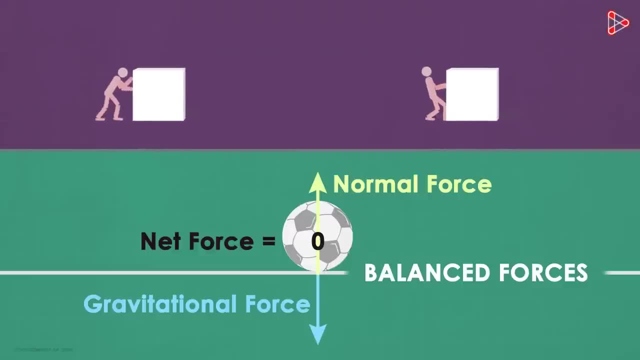 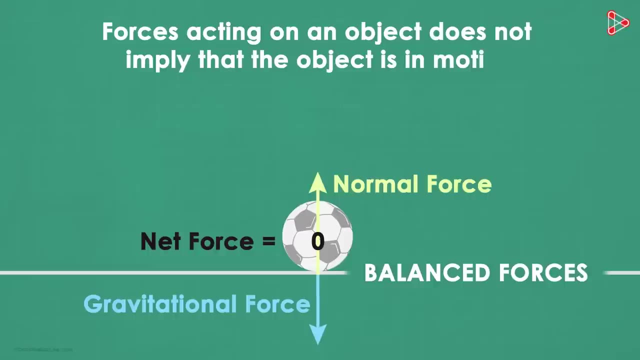 So what does this tell you? Just humans? pushing or pulling is not the only kind of force. And just because there are forces acting on an object will not mean the object will move. For the object to move, there has to be some net force. 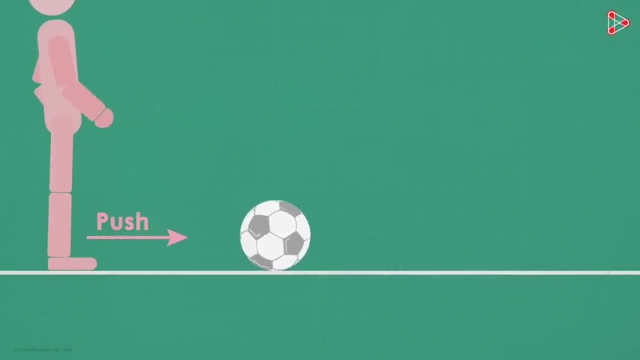 So now, let's say a person softly kicks the ball. What happens then? Yes, the position of the ball changes. Why did the position change? It's because there was another magnitude of force acting on it, and this time the forces were not balanced. 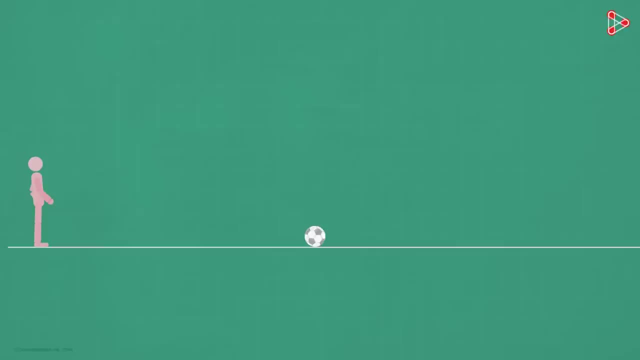 The ball moved and there was displacement, But hold on. Why did the ball stop moving? after covering 15 meters, The ball started moving at a pace and then slowly came to a halt If there is no force from the other side to stop it. 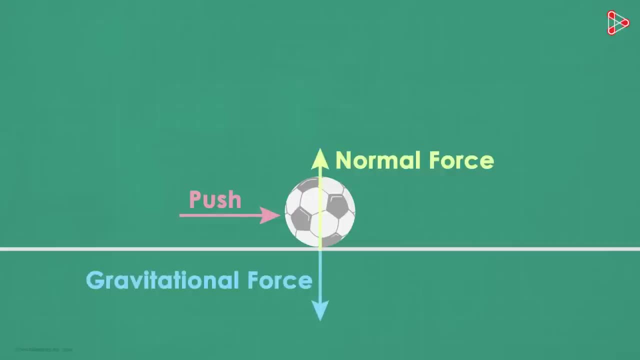 how did it stop? Was there a force which stopped it? Yes, it was friction that stopped the ball. While the force you applied was towards the right, the force of friction was towards the left. Let's make it even more interesting. Assume your screen to be a frame of reference in this example. 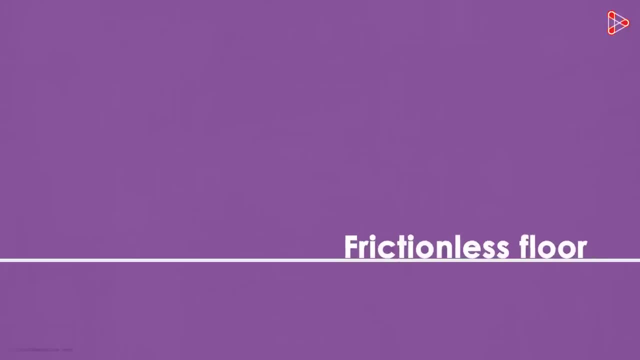 Also assume that this straight horizontal line is a frictionless floor and there is no air resistance. The ball appears from the left of your screen and moving towards the right at a uniform velocity of 2 meters per second. The only two forces acting on the ball are the gravitational. 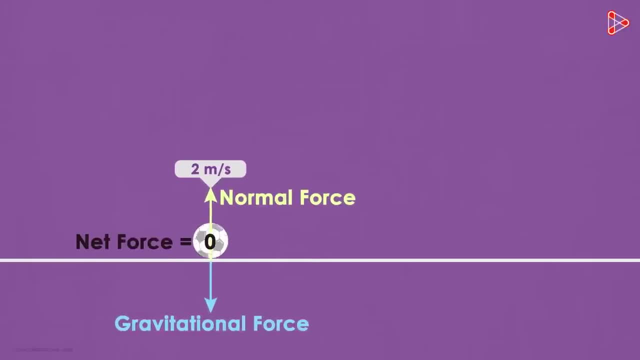 and the normal forces which net each other out In this setting. will the ball ever stop moving? No, it won't. It will continue to move along the same path, at the same speed, unless there is another external force which acts on it. 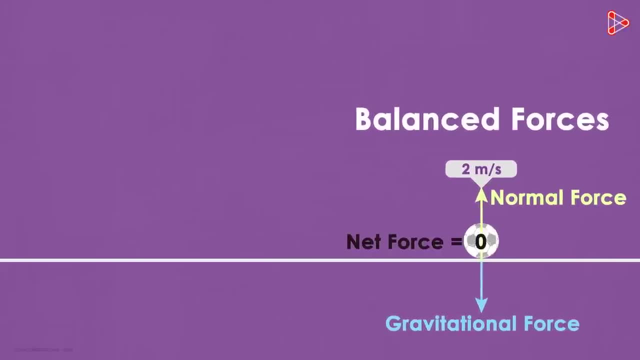 Here. as the forces are balanced, the ball will continue to move at 2 meters per second. Most people assume that if the external force is moving, then there is some net force acting on it, but that's not true. An object will continue to move at uniform velocity.